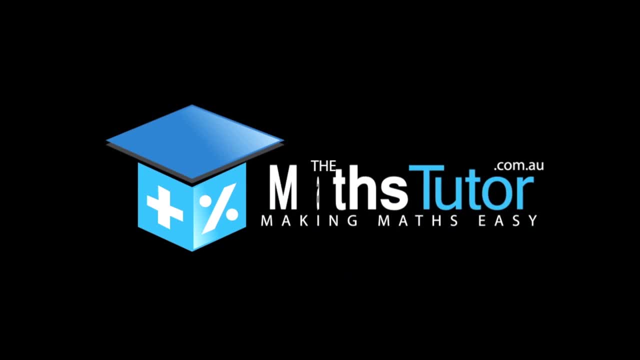 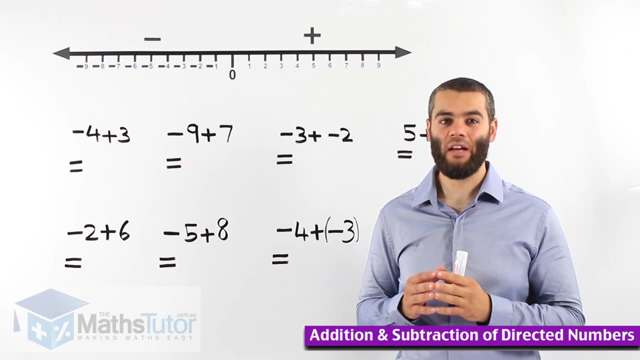 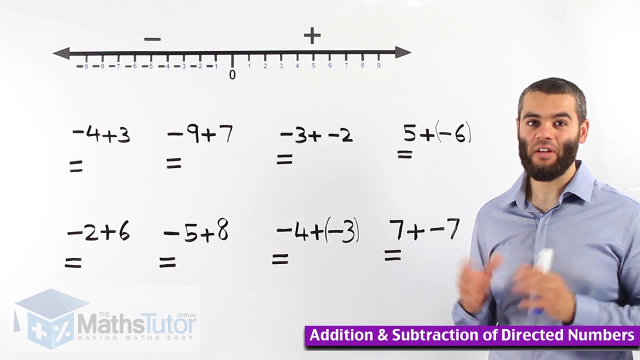 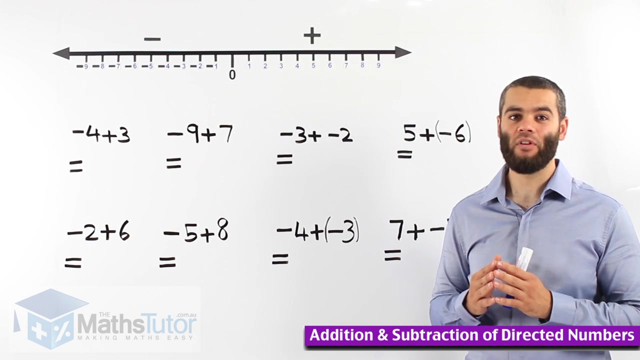 Hey guys, in a previous lesson we learned about the number line extended after the zero and we've introduced what we have, or what we call as negative numbers. Now we're going to use the number line to learn how to add and subtract directed or negative numbers. Now, at the start, 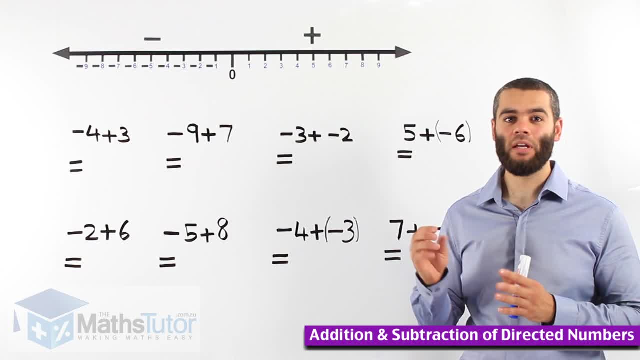 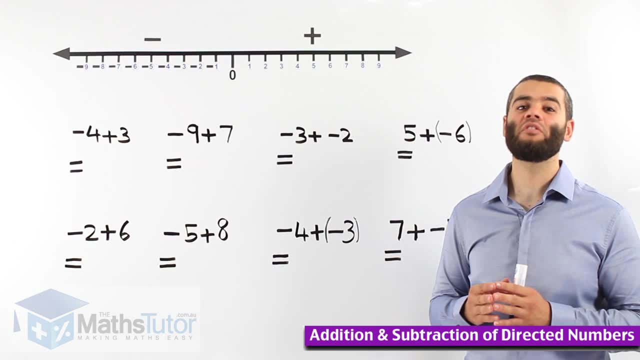 you're going to use the number line, but after you get the hang of it you're going to become so quick and so good that you're not going to use the number line at all. But it's always good. always tell my students for the first couple of times that you are using and you 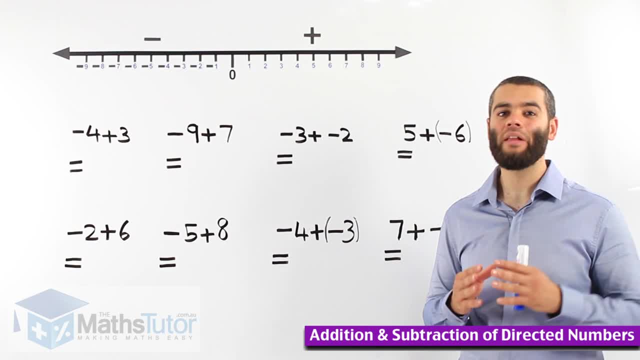 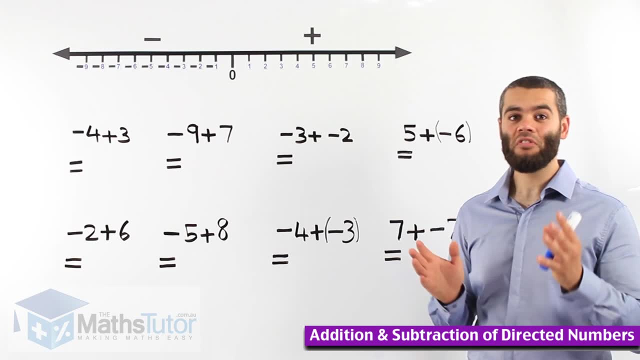 are working with these questions, even if it takes you one whole exercise, or 15 or 20 or even 30 to 40 questions that you need to do using the number line, there's nothing wrong with it. use it and after you get the hang of it, you won't need the number line again. 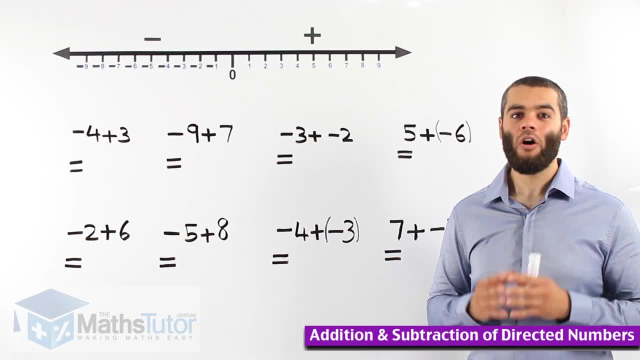 But for the start let's use the number line to get an understanding of how it actually works. Here we have questions, and these questions involve negative or directed numbers. We're going to go through one by one and you're going to see it's a very easy process using. 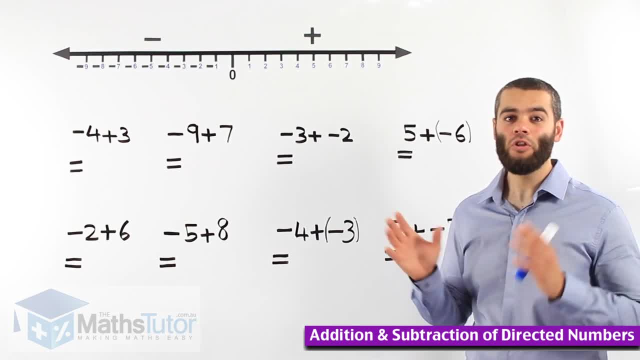 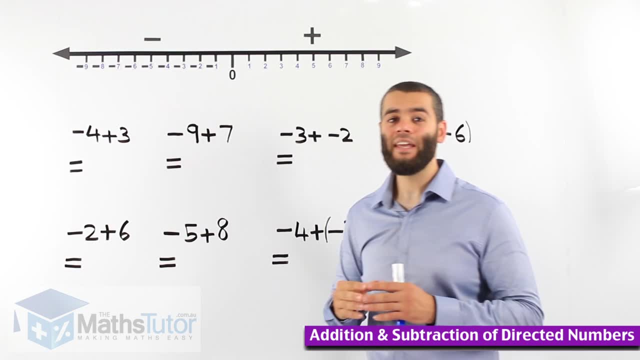 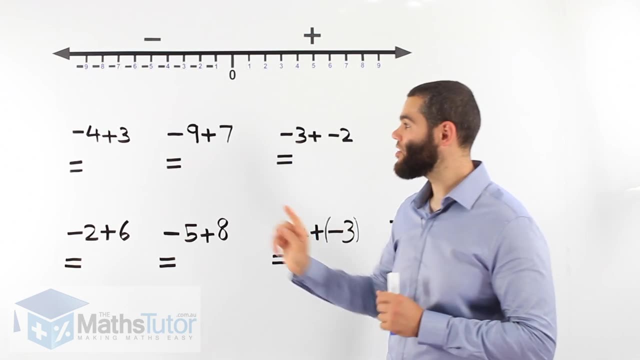 the number line and hopefully by the end of the lesson you can probably even do them without a number line as well. Okay, let's start. We have this question saying negative 4 plus 3, negative 4 plus 3.. What we do? we use the number line. we start at negative 4 so we can put our pen or our finger on. 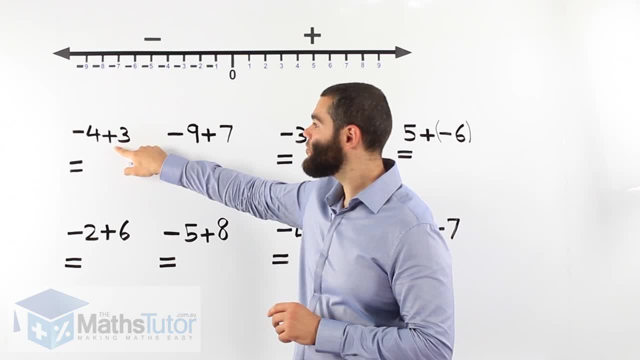 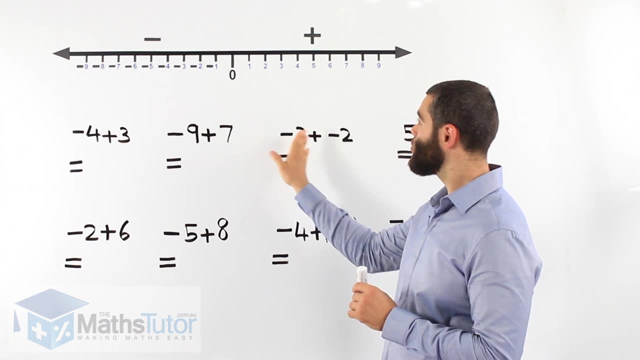 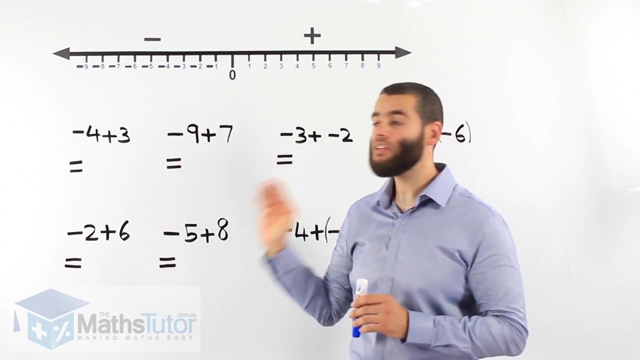 negative 4. there it is and it says we have to add 3.. Now a quick rule to remember: when we're adding, we're moving towards the right, we're moving towards the addition, we're moving towards the plus direction, and if we're minusing or we're taking away, we're going towards the 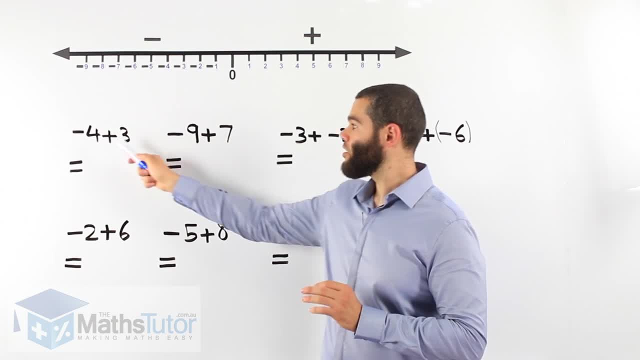 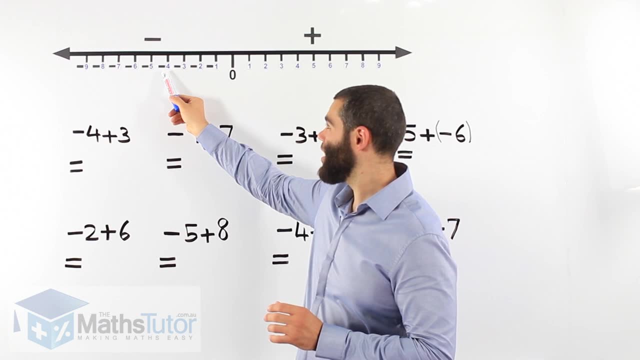 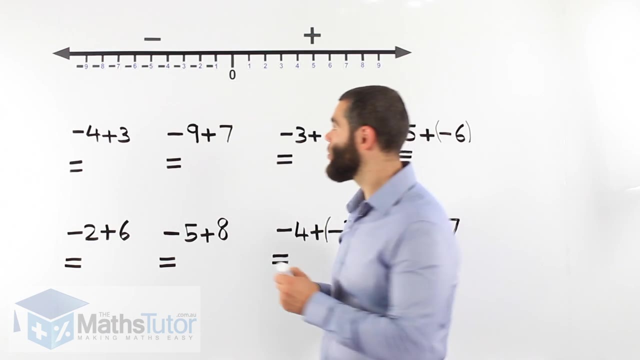 left. That's very important. So negative 4 plus 3.. We start at negative 4 and we add 3. we're going to the right because we're adding 1,, 2, 3.. Our answer is negative 1. We start at. 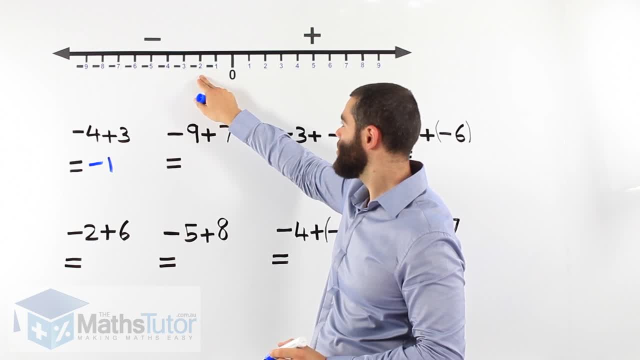 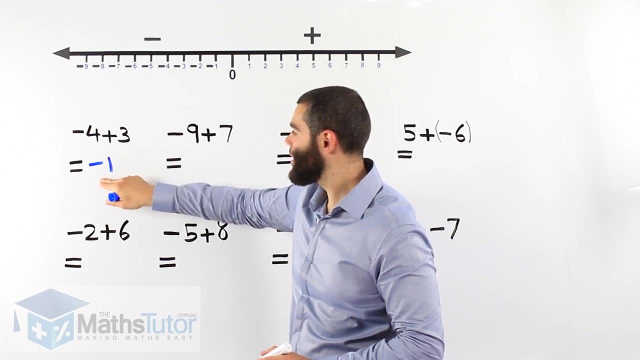 negative 4 add 3, 1, 2, 3.. As you can see, I'm counting the moves: One move, two moves, three moves. So negative 1 is our answer. Then we have another example: minus 2 or negative. 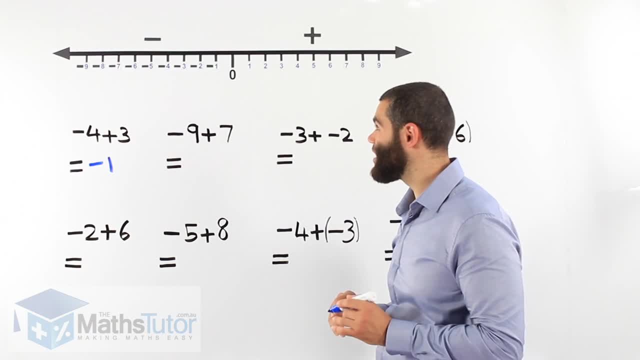 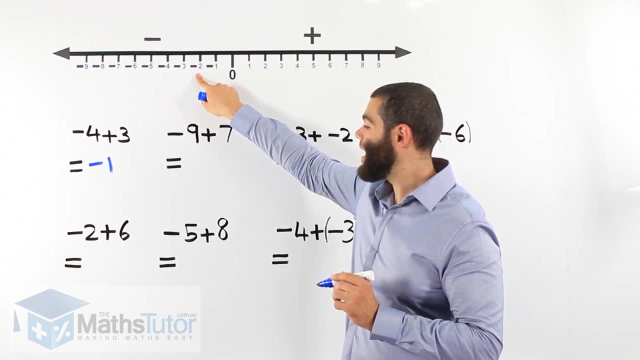 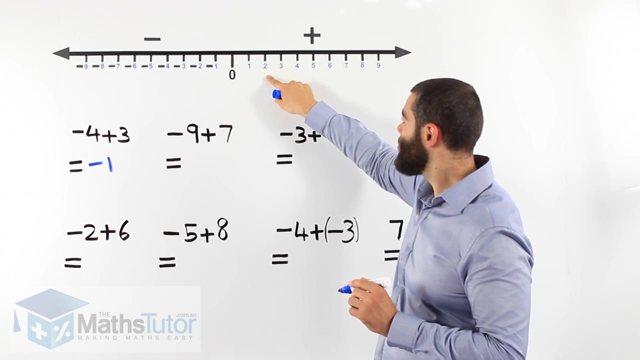 2 plus 6.. What do we do? first, We start at negative 2.. Negative 2: we're adding 6.. Addition meaning we're going towards the right. So we're adding 6, 1,, 2,, 3,, 4,, 5,, 6.. So our answer: 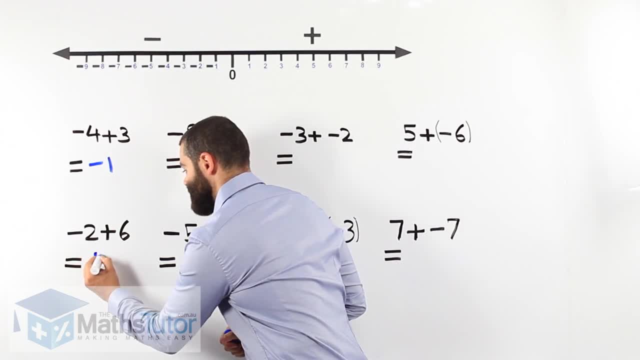 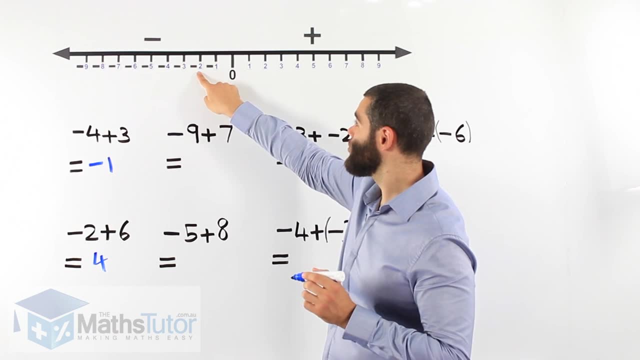 is positive 4.. We don't need to write positive, we just write 4, because we know 4 means positive 4.. And notice, when I was counting, I started from negative 2.. I said 1, 2. I had to ensure. 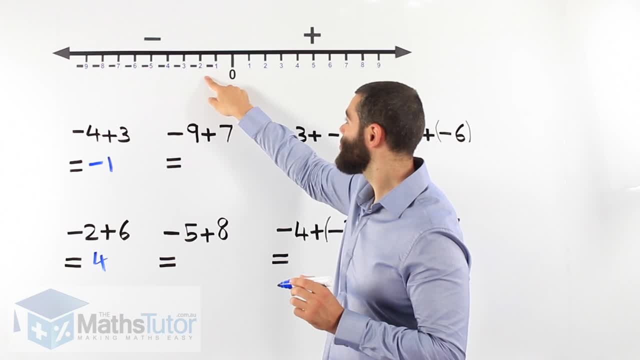 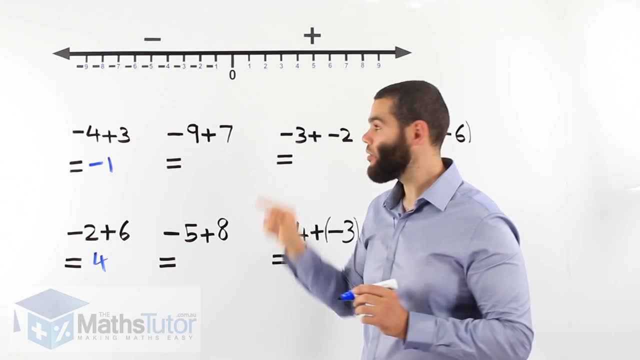 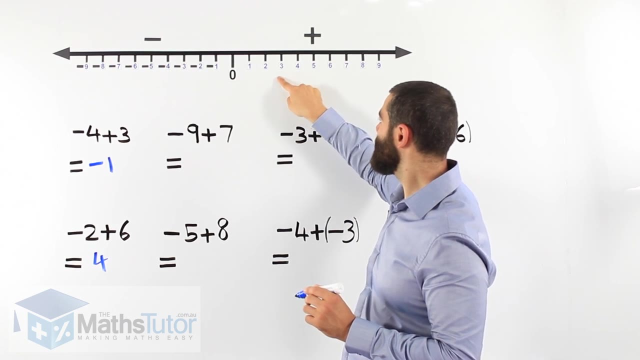 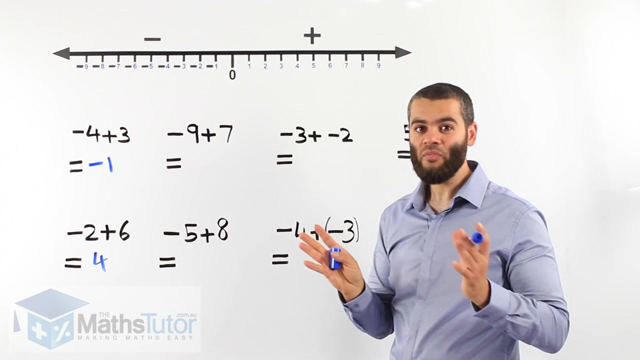 that I had the 0.. I've seen students make a mistake where they just move and they go straight to the other side, forgetting the 0.. Very important: The 0 is a number. we need to add it part of the process. 1,, 2,, 3,, 4,, 5,, 6.. Our answer is 4.. Let's see if you can do this one. Where are we? 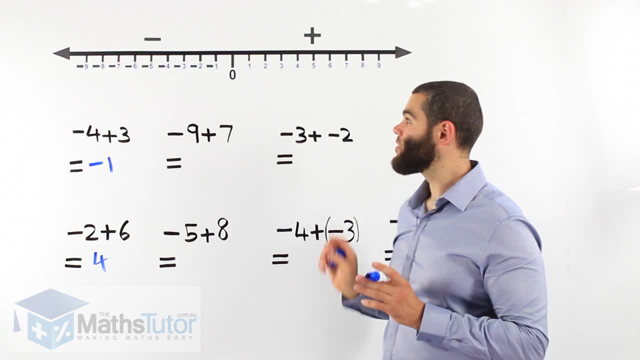 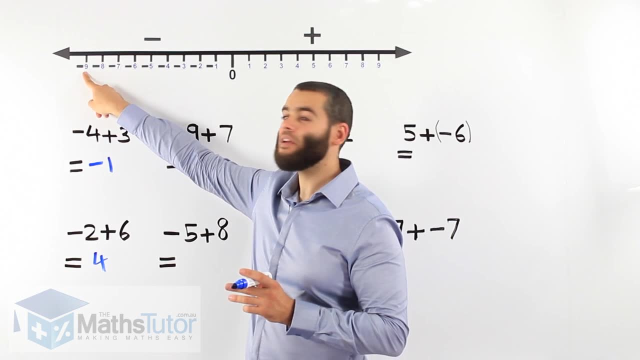 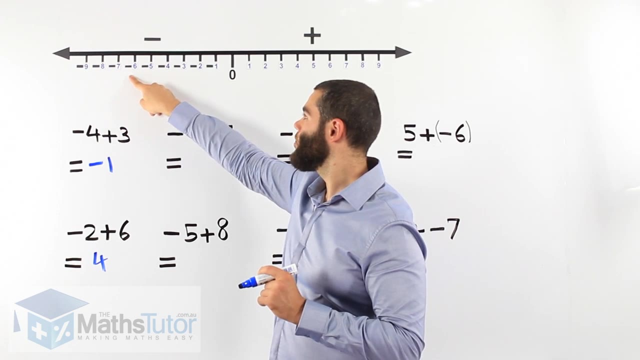 going to start At negative 9.. So negative 9, it says negative 9 plus 7.. So we start at negative 9.. Add: we're going towards the right and we're going to add 7.. 1,, 2,, 3,, 4,. 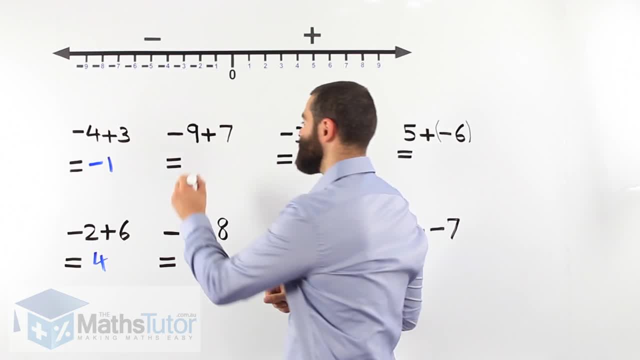 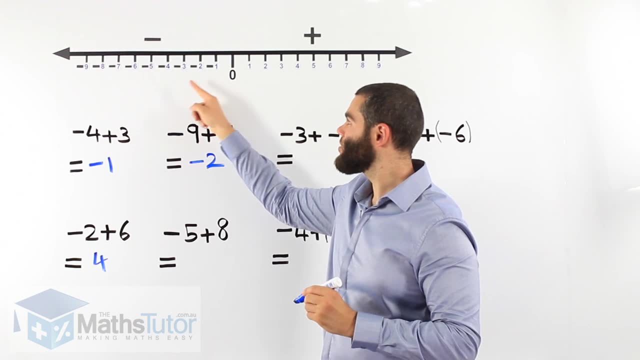 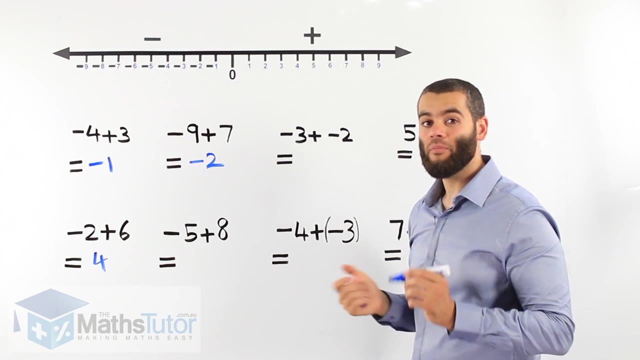 5, 6, 7.. So our answer is negative 2. Negative 9, moving 7 times, we end at negative 2. Minus 5 plus 8. Again, we start at negative 5 or minus 5.. Negative 5: there we're adding. 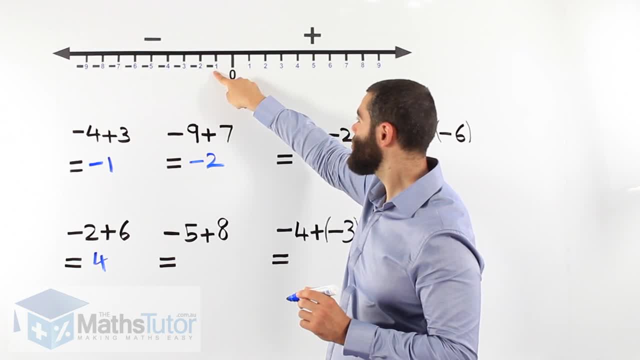 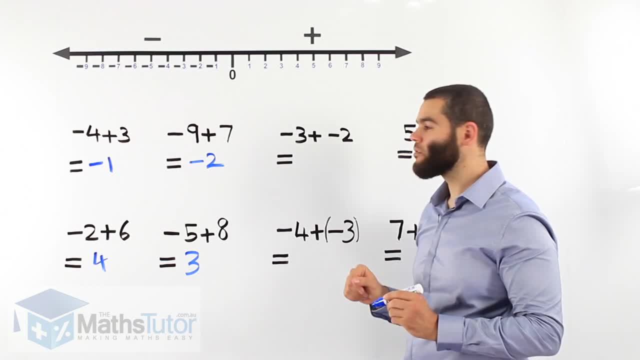 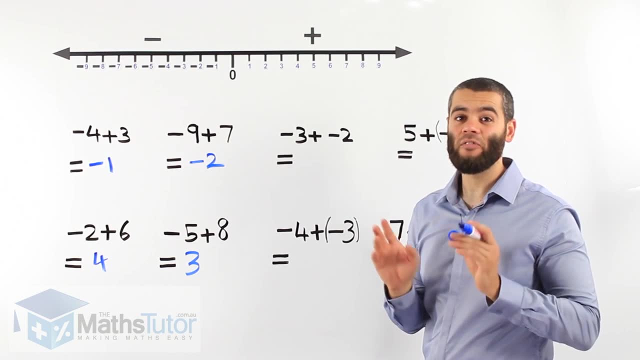 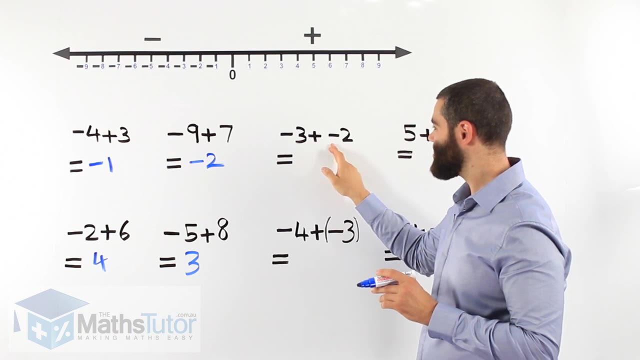 Now we have something a little bit different. We have negative 3 plus negative 2.. Negative 3 plus negative 2.. Okay, what do we do here? We have a plus and a negative. Whenever we have a plus and a negative next to each other, side by side. 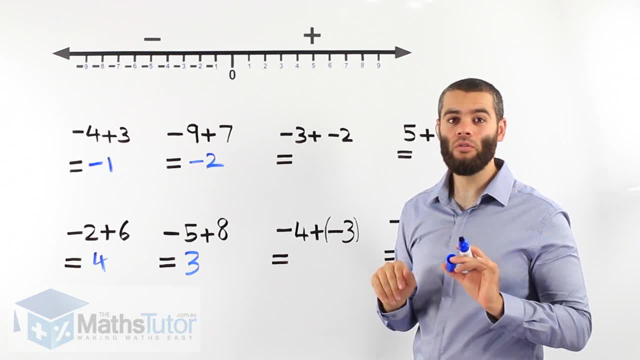 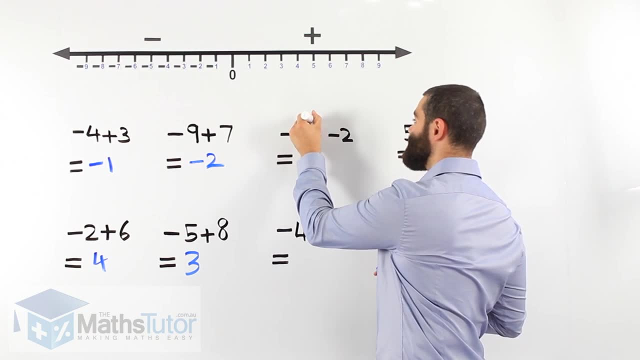 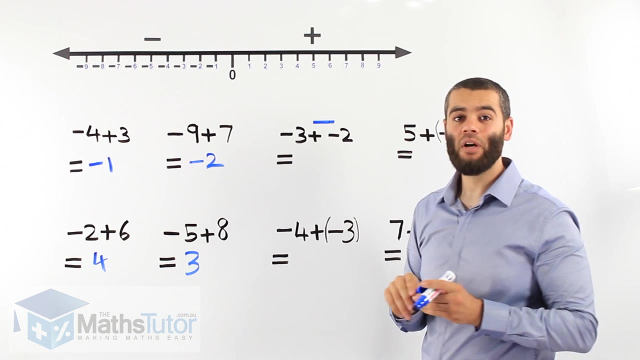 they don't like each other. they don't like each other at all. so what do they do? they have a big fight. they have a fight and they always the negative will always win, the negative will always win. so whenever you see a plus and negative next to each other, like that side by side- they 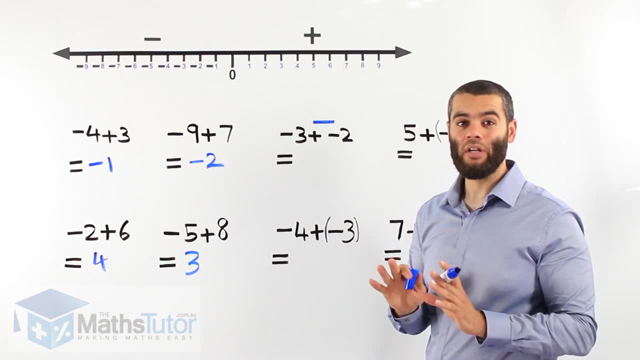 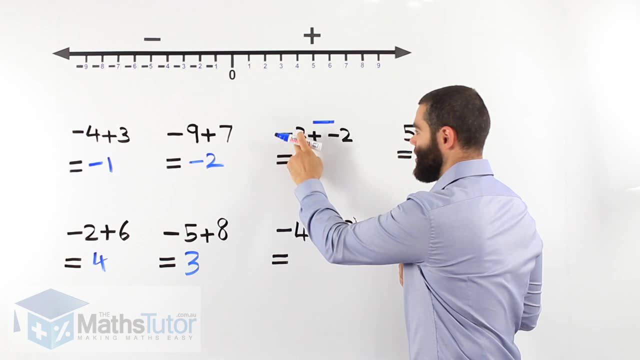 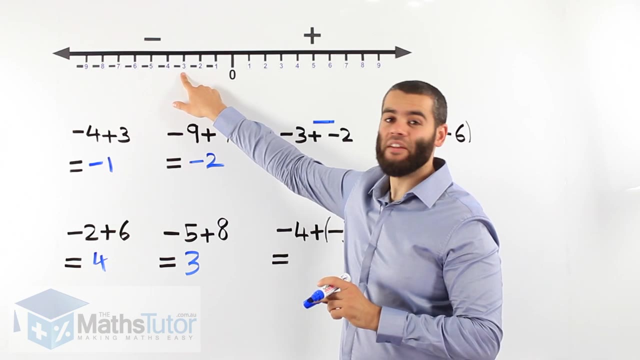 don't like each other. they have a big fight and negative will always win. so how do we do it? now? it becomes negative three minus two, negative three minus two. so we start at negative three and we minus. now we said positive or we addition, we go to the right minus. of course we're going to go to the 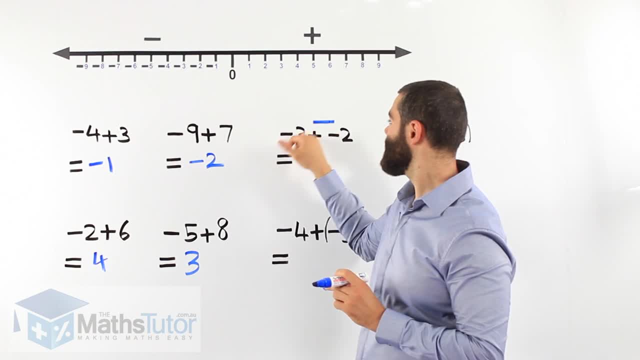 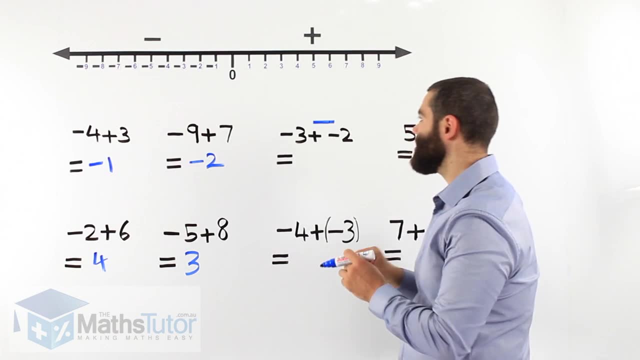 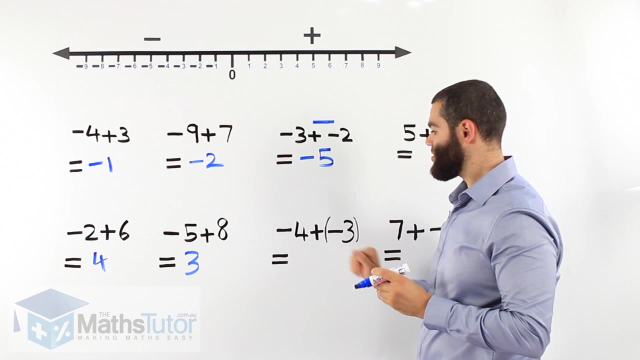 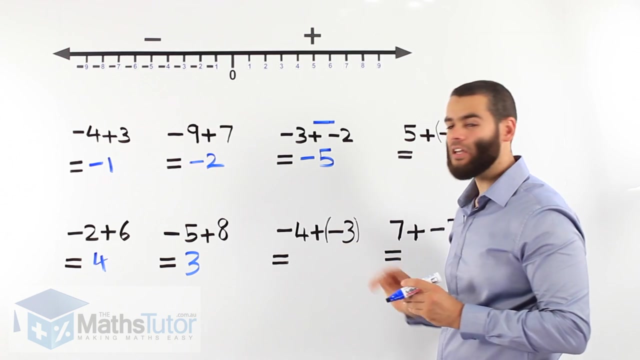 left minus three minus two, or negative three minus two minus three minus two, one, two. our answer is negative five. the number is getting smaller once again. negative four plus in brackets. negative three. now the brackets don't get confused, it's exactly the same as the top, so don't get confused because the brackets are there. it's just telling us. 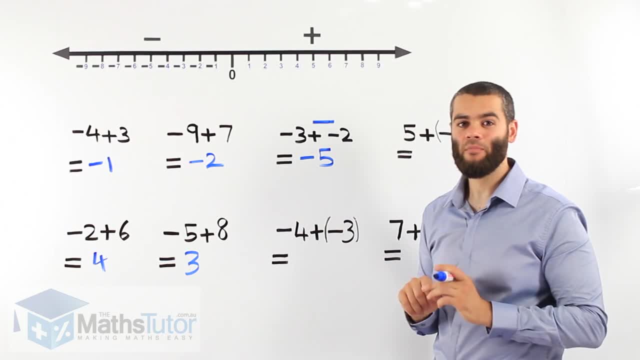 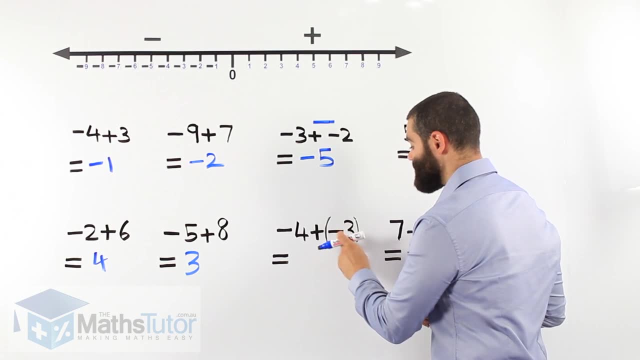 that there is a plus and a minus, just to distinguish them. sometimes you'll see the brackets, sometimes you don't. however, disregard them. Minus 4 plus minus 3, plus minus. we said they don't like one another, they have a fight. 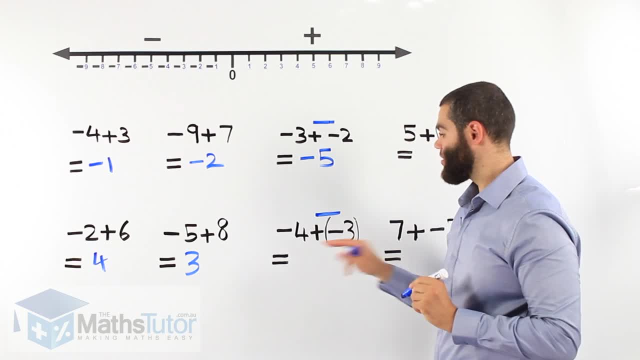 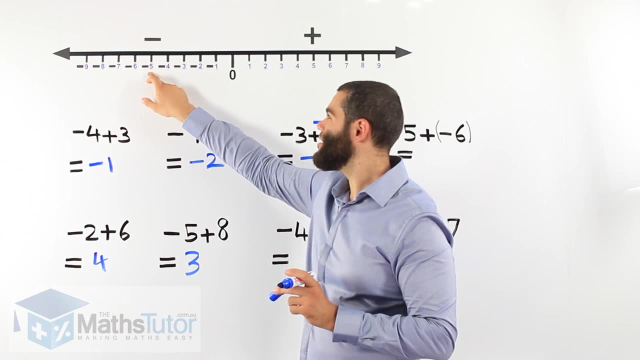 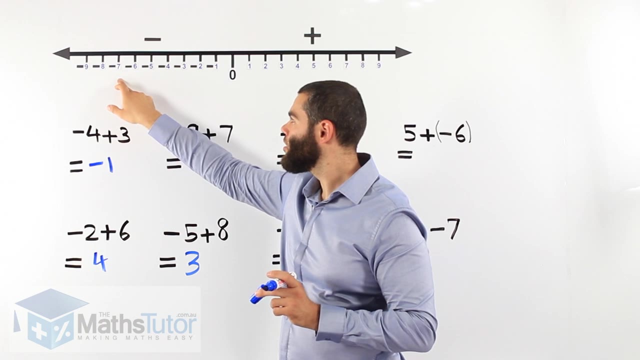 so, and always minus will win. So minus 4,, minus 3, we start at minus 4, and we go back: 3, 1,, 2, 3, start at minus 4,, 1,, 2,, 3.. 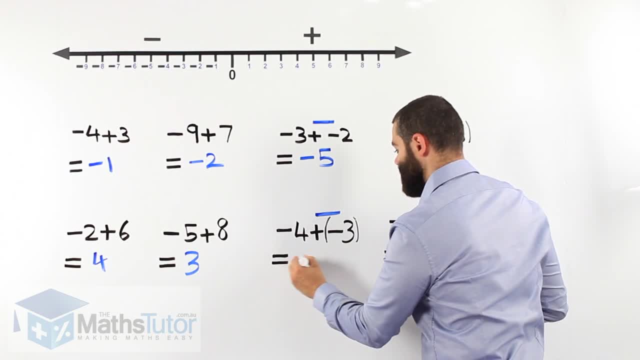 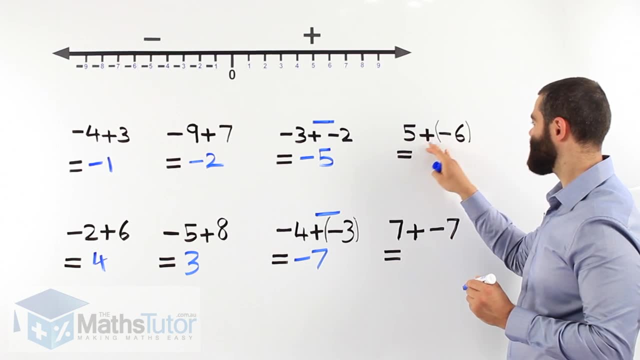 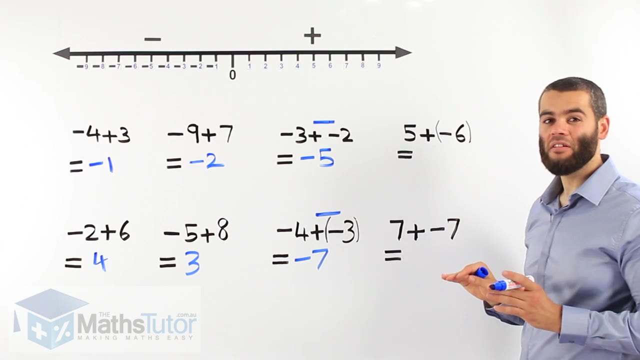 So our answer: negative. 4 minus 3 is negative 7.. Another one: 5 plus negative 6 in brackets. we said we disregard the brackets here we notice a plus and a minus. we know what do they do. 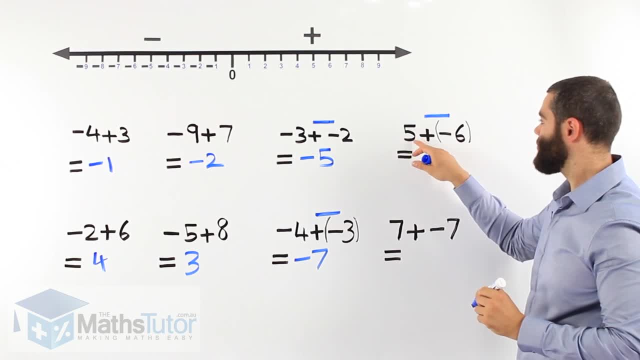 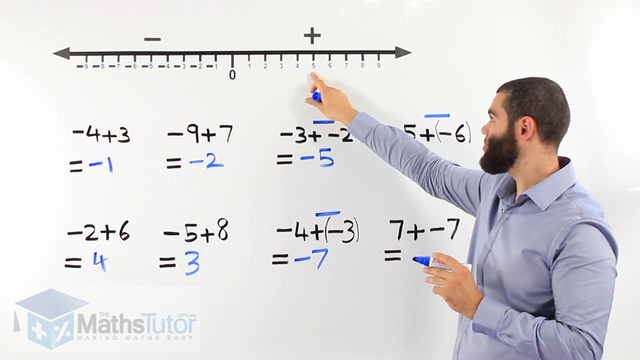 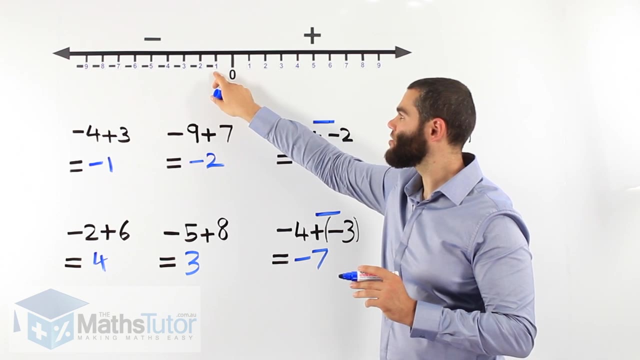 They have a fight and the minus wins. So 5, take away 6, we start at 5, notice it's a positive 5, so we start at 5 in the positive. Next side minus 6,: 1,, 2,, 3,, 4,, 5, 6, at negative 1.. 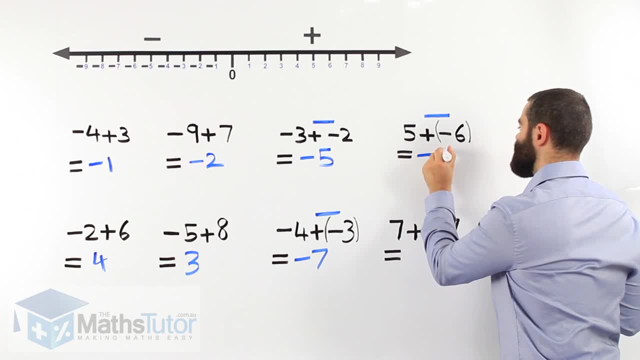 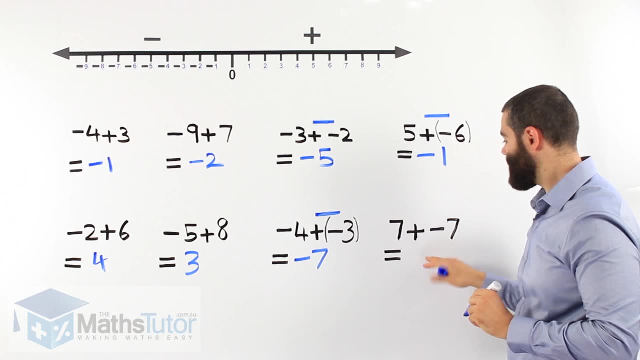 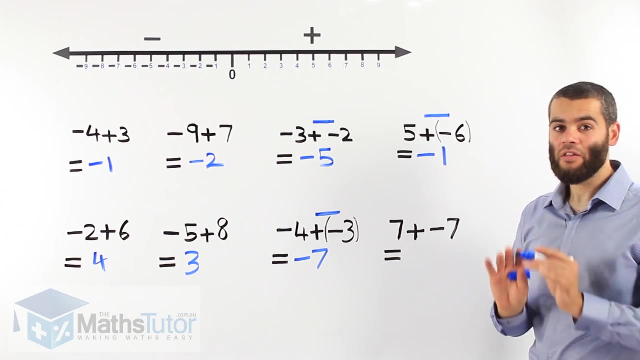 So we go to the left because we're taking away and our answer is negative 1.. 5, take away, 6, is negative 1.. Then we have 7 plus negative, 7.. Again, a plus and a minus. next to each other. they don't like one another, they have a fight. 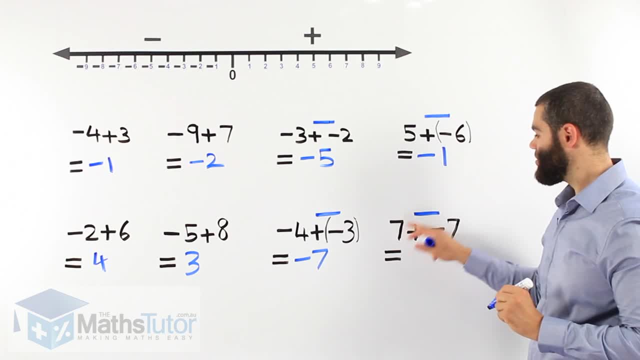 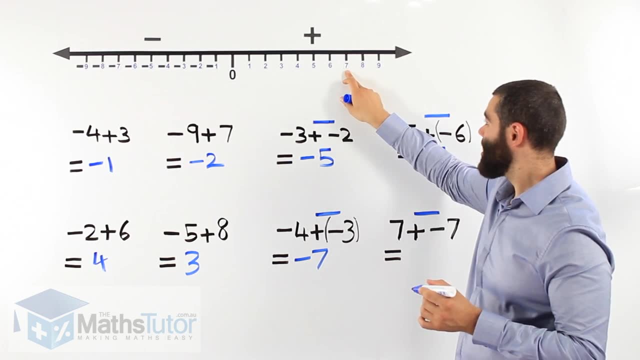 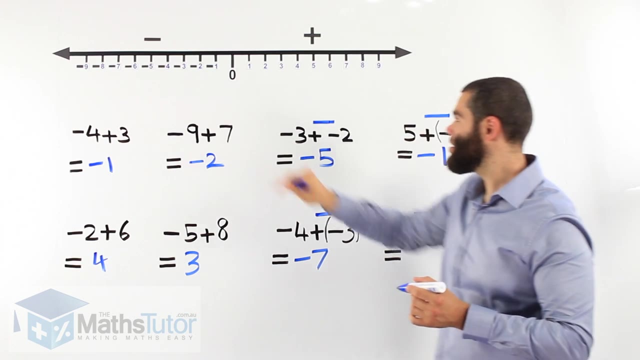 minus will always win 7, take away 7, I mean it's too easy, but we'll still use the number line. we start at 7, minus 7, so 1,, 2, 3, 4, 5,, 6, 7, obviously our answer is going to go and become nothing. 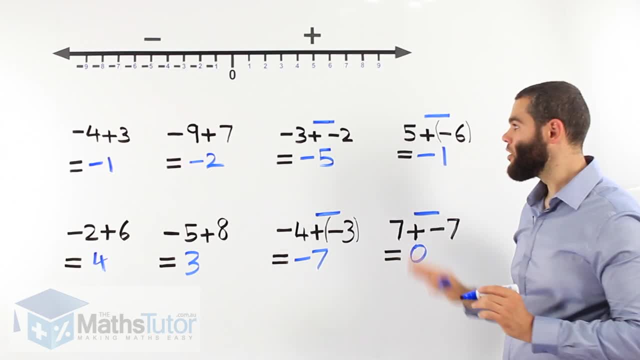 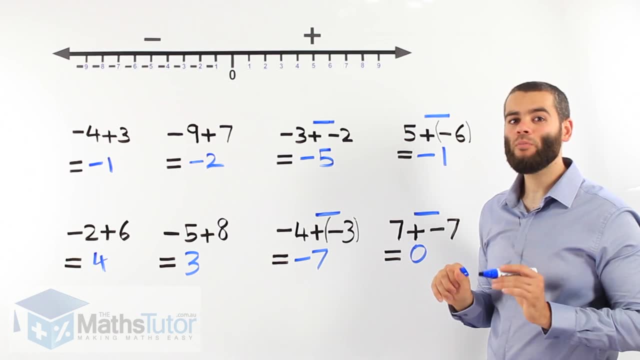 0, 7,. take away 7, is 0.. So this is the basics of how to use a number line to add or subtract directed numbers. Next we're going to do a formula. A couple more examples. that way you get the hang of it and by now you should already. 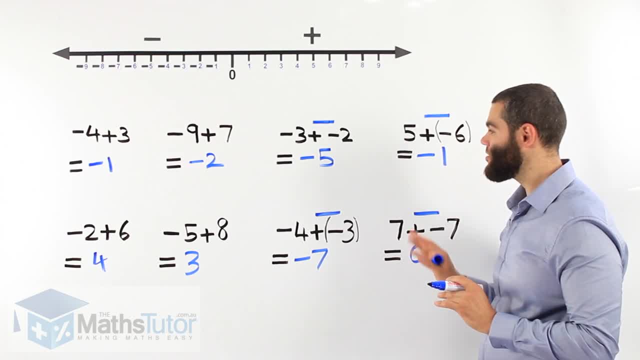 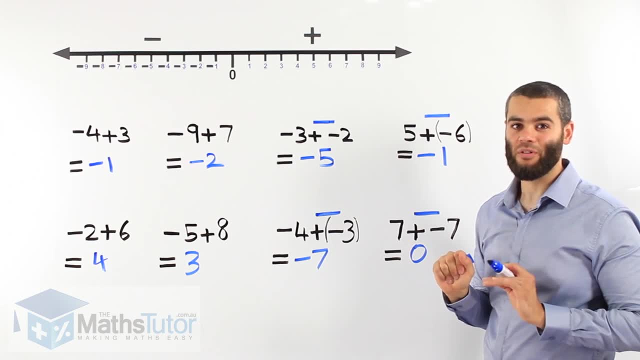 have a very good understanding of how to solve these number sentences using the number line and hopefully you probably even now see the pattern where you don't even need the number line at all. Now that we know how to use the number line, we can actually solve a little bit more harder. 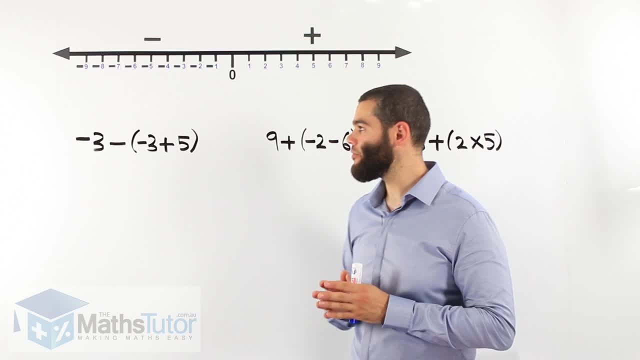 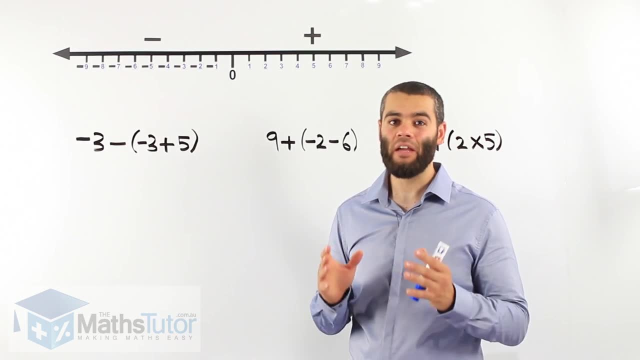 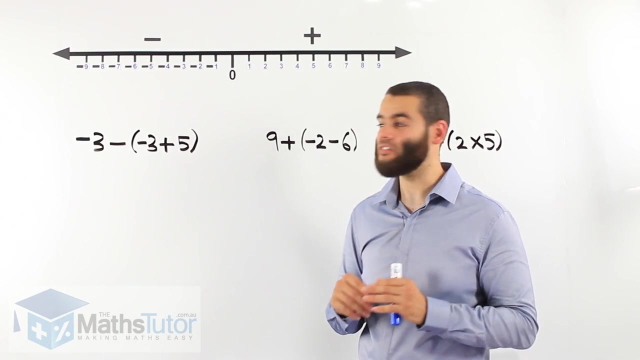 questions. Let's see how they're done. In this example we have negative 3 minus and in brackets negative 3 plus 5.. We know that we have to use brackets of division, multiplication, addition and subtraction. We still have to follow that order in all our number sentences. 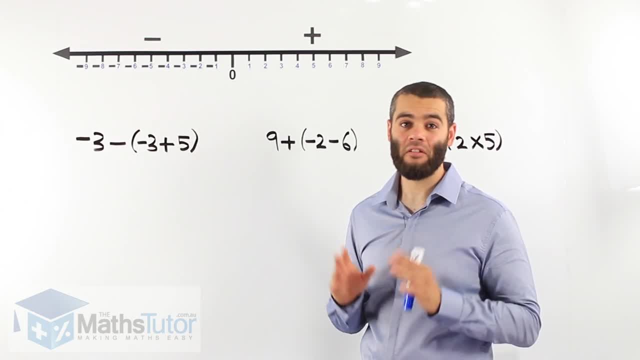 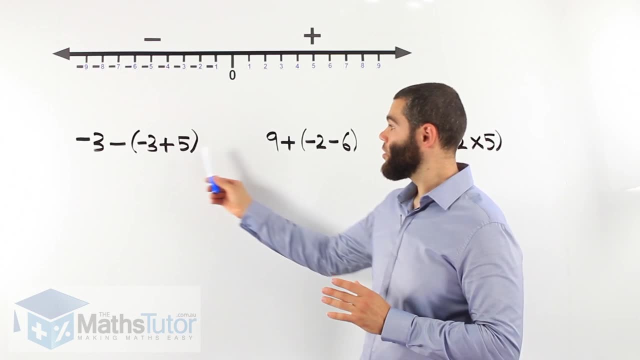 Now here we notice we have brackets, so we have to complete what's in the brackets first before we go outside. In the brackets we have negative 3 plus 5, so using the rules, negative 3 plus 5, where? 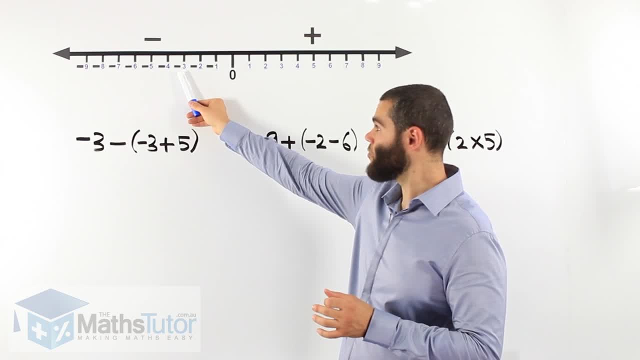 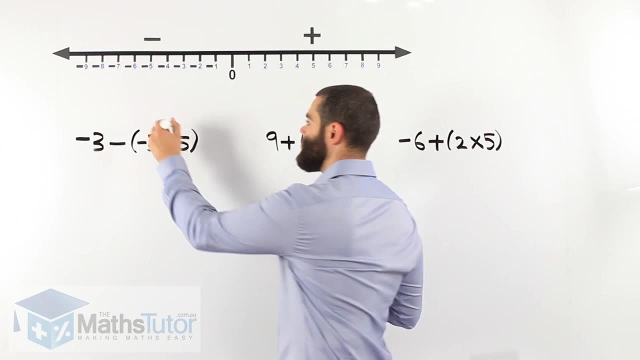 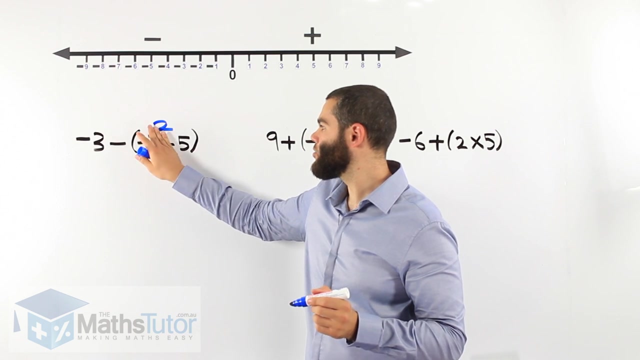 do we start? We start at negative 3.. We add 5, we're going to the right: 1,, 2,, 3,, 4,, 5, our answer is 2.. Now, negative 3 minus 2.. 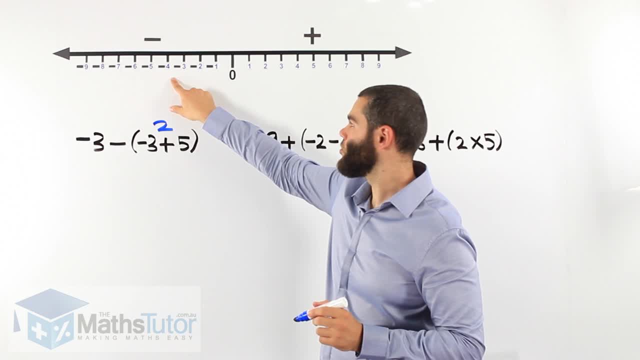 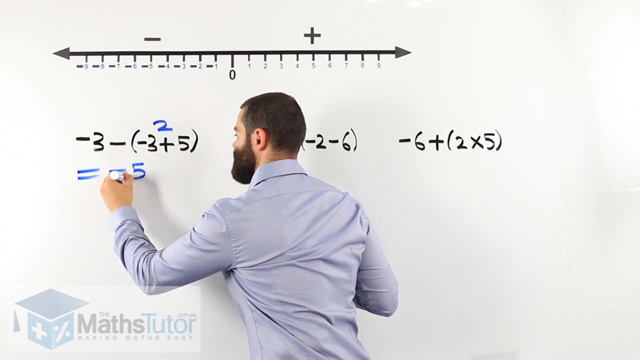 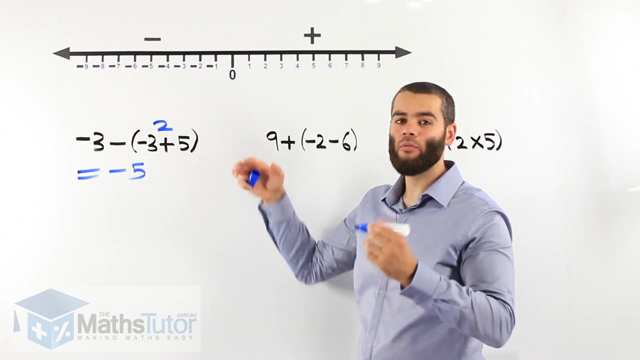 We start at negative 3, and we minus 2,, 1,, 2,. so our answer in full: negative 5.. Minus 3 minus 2 is negative 5.. We start from the brackets, We move on. 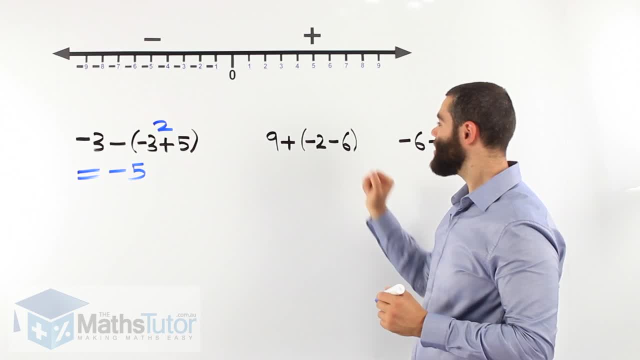 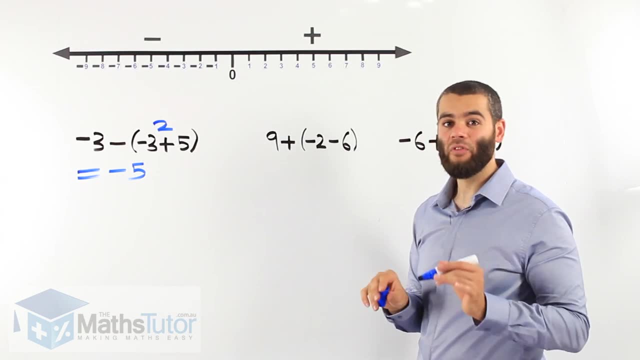 Here we have 9 plus in brackets, negative 2 minus 6, close bracket. So we follow the order of operations which says that we have to do the brackets first To do that negative 6 minus 2 minus 6.. 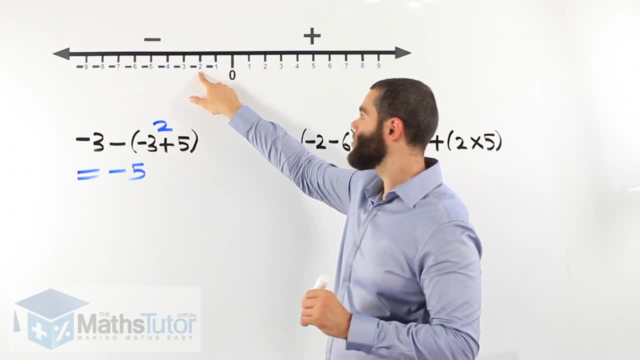 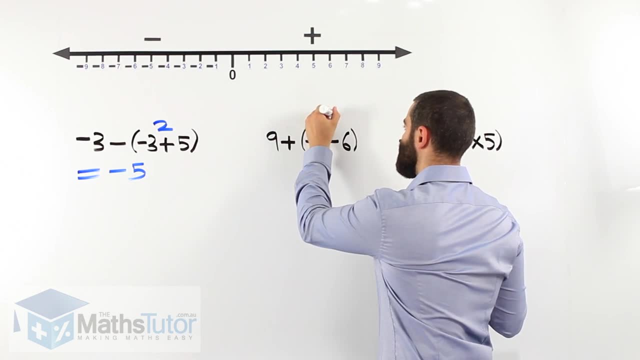 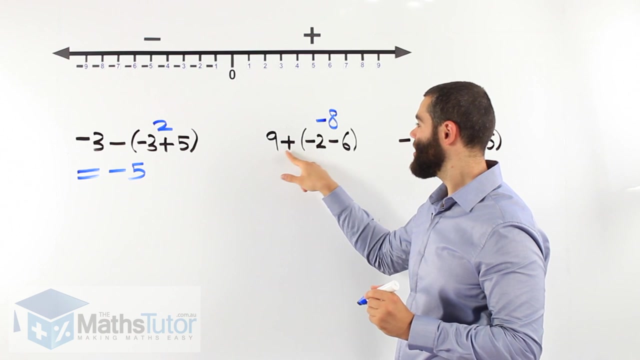 We start at negative 2, and we minus 6,, 1,, 2,, 3,, 4,, 5,, 6.. So negative 8.. Then 9 plus negative 8,, 9 plus negative 8.. 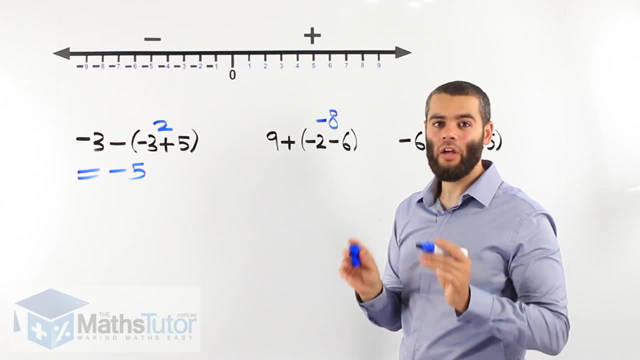 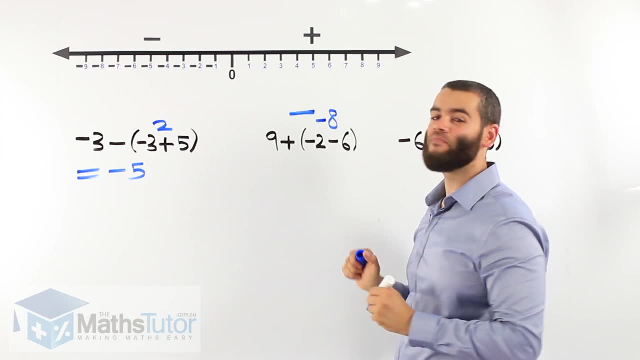 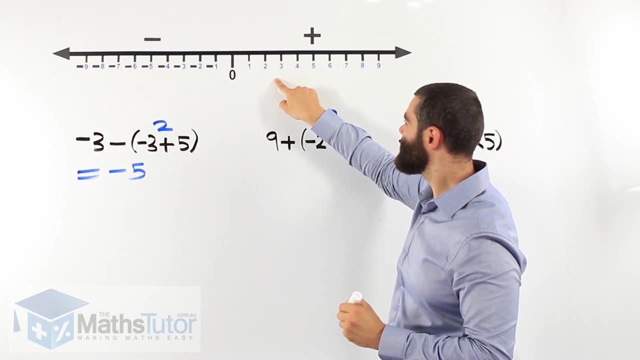 We notice a plus and a minus next to each other and we know they don't like one another. They have a fight. Minus will always win. So it's 9 take away 8, 9 take away 8,, 1,, 2,, 3,, 4,, 5,, 6,, 7,, 8.. 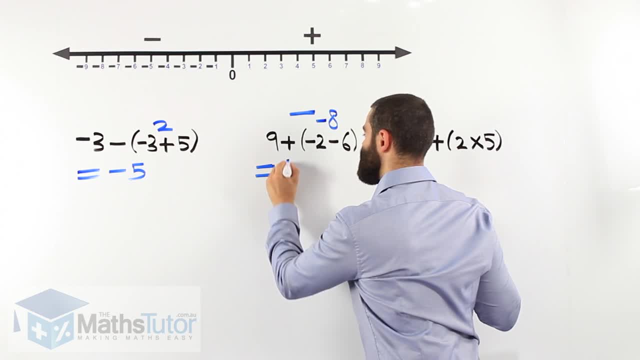 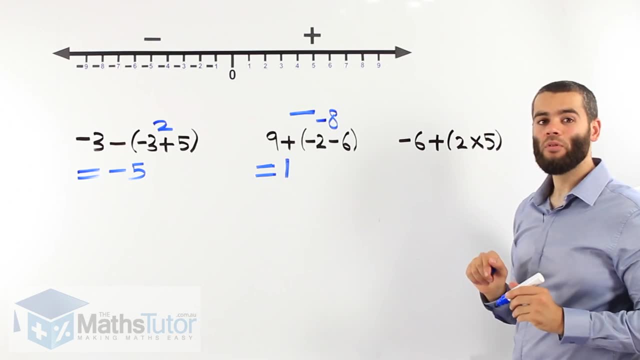 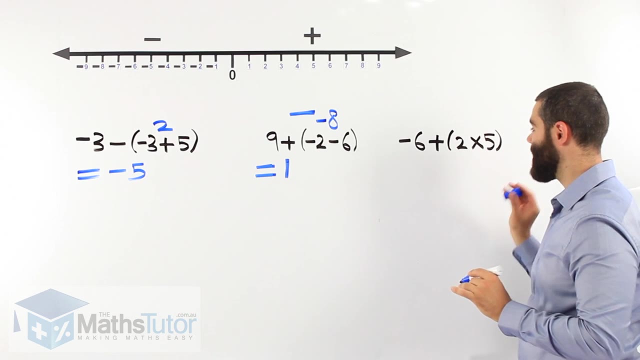 Of course the answer is 1.. 9 take away 8, our answer here is 1.. One last example: Negative 6 plus in brackets 2 times 5.. Again, order of operations states we have to complete the brackets first.